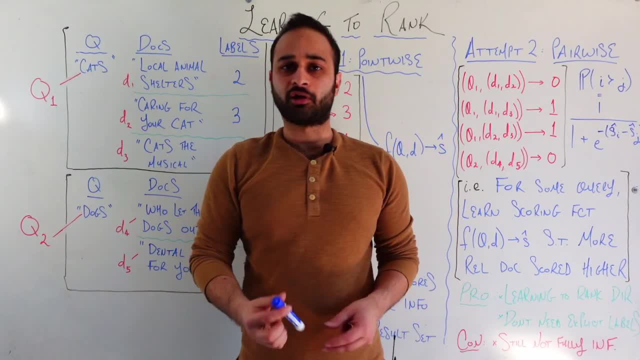 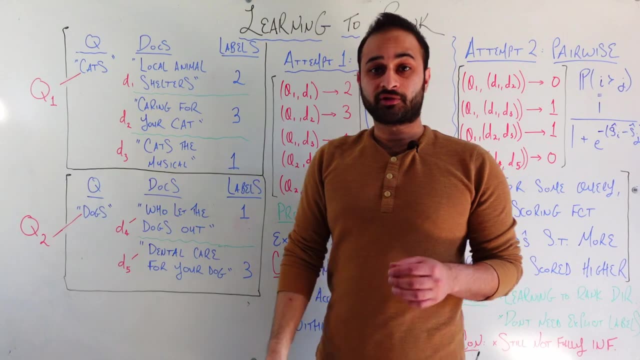 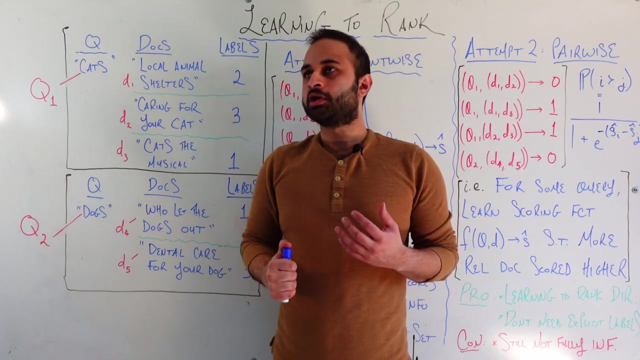 call D3. And this cat's query will be called Q1, which is query one. So we have these three possible results for this one query. and the last part of the story for this query is the labels. The labels in learning to rank have a very special place in my heart because they are interesting. 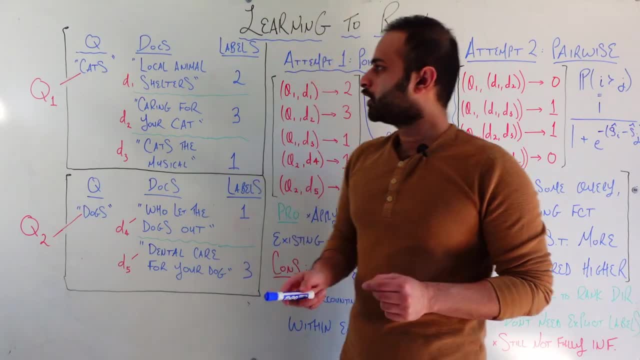 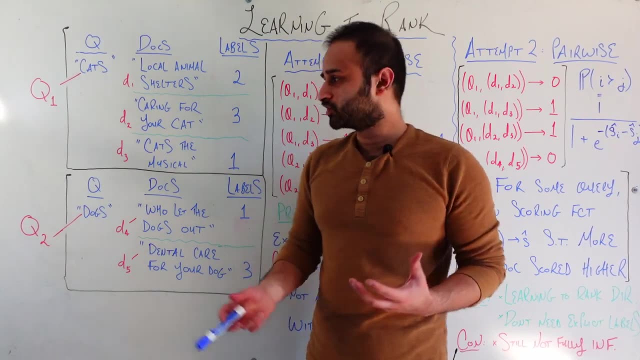 they're known to a lot of bias, but we'll touch on a little bit of that here. First of all, what are the labels? The labels are simply some kind of score, some kind of gauge about how relevant each of these documents is for this particular query, For our labels today. 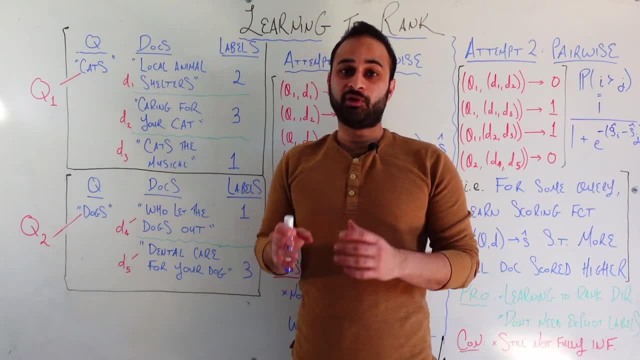 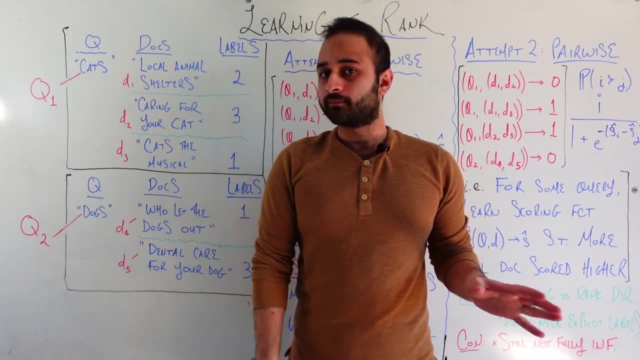 we'll be assuming they're either 1,, 2, or 3,, with 3 being kind of signaling that this document is really, really relevant to this query, and 1 meaning that it's not relevant at all. So we have these labels here and the immediate question is: where do I get those labels? 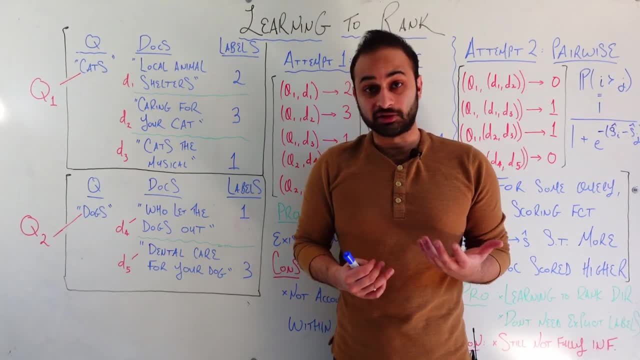 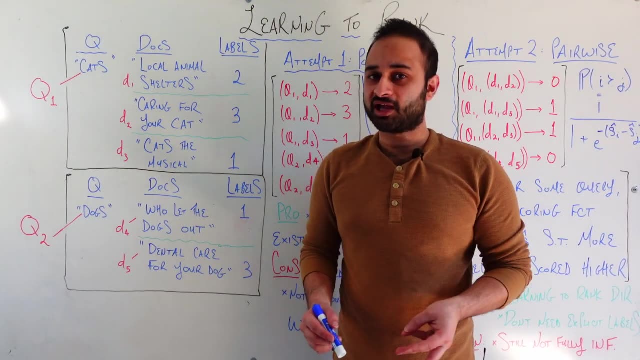 The labels can come from many different places. At the ideal level, they are given to you by your users. They're just hand-labeled. Obviously, that takes a lot of resources, time and money together, so most of the time for any real learning to rank they're gathered via some kind of 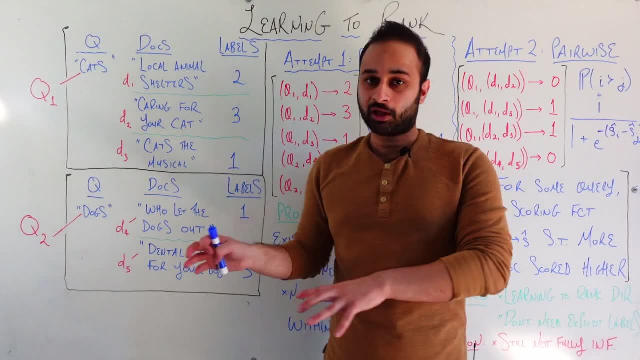 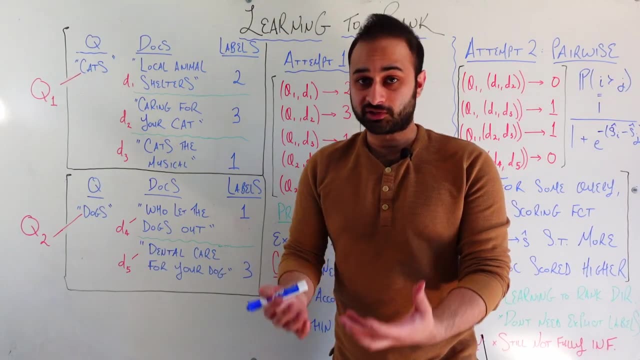 automated system. For example, if you actually have the search engine running, you can use the clicks on these things as your labels. The more clicks something gets kind of says that it's more relevant, and the less clicks, the less relevant. There are issues. 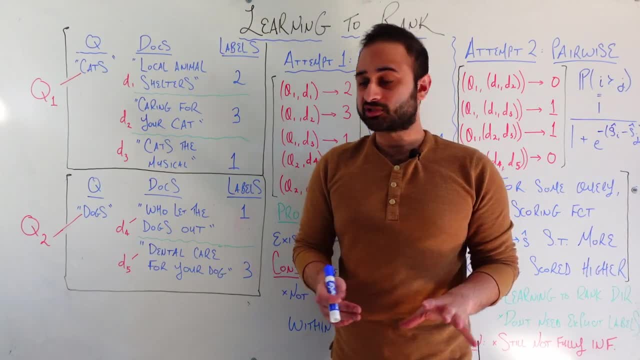 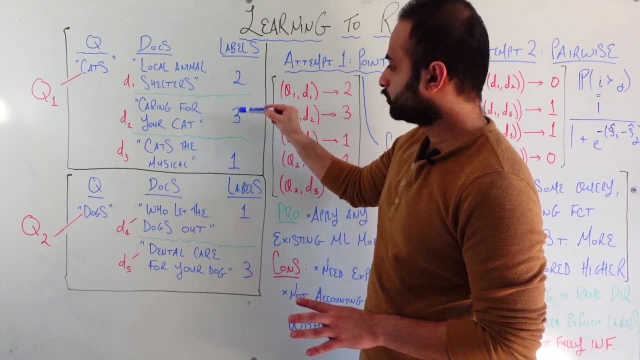 in that. but we won't get into that. We'll just say that we have some kind of labels and the higher the label, the more relevant this document is to the particular query in question. So we have labels 2,, 3, and 1 here And we have our second query, dogs, called q2.. 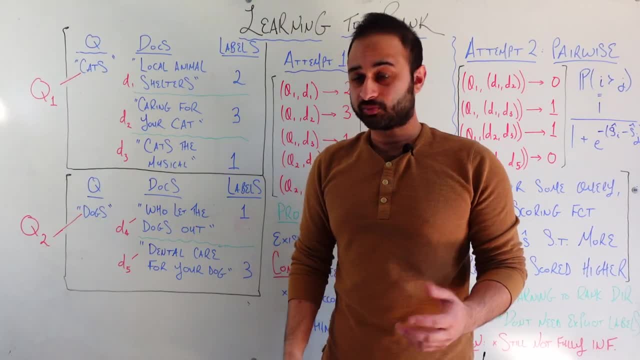 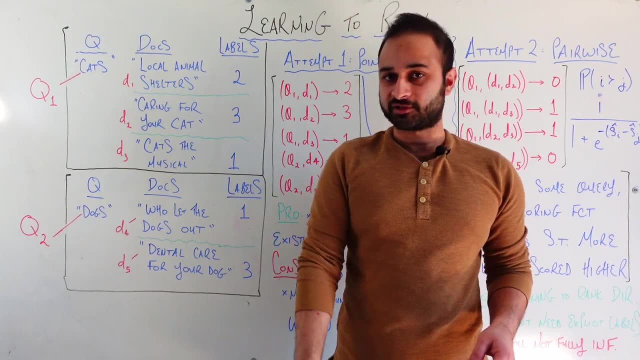 This one happens to just have two documents that are irrelevant to it. possibly. We have who let the dogs out, and we have dental care for your dog, the first one being not relevant and the other one being very relevant. So this is the data, so to speak, for our learning. 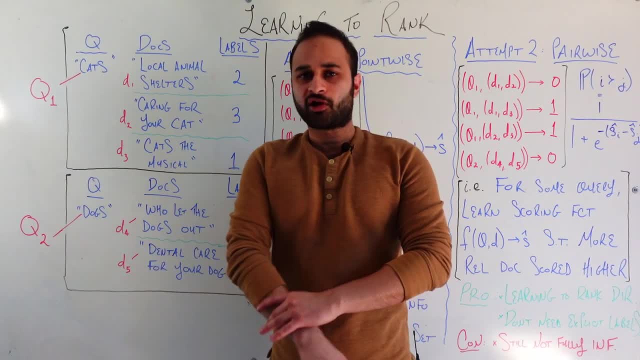 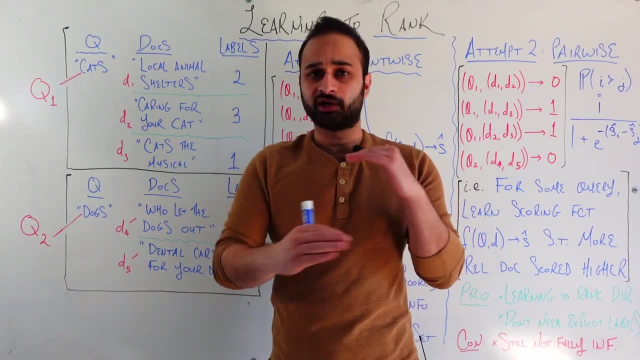 to rank problem. This is the raw data. Now, how do we go from this raw data and kind of reformat it so that we can actually learn something, so that we can learn which documents should be ranked above others for a particular query? We're going to start with the most naive approach. 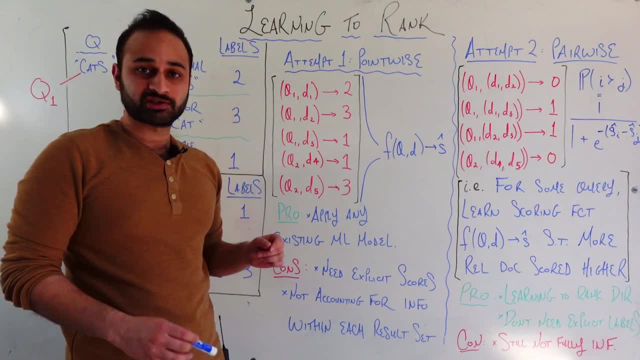 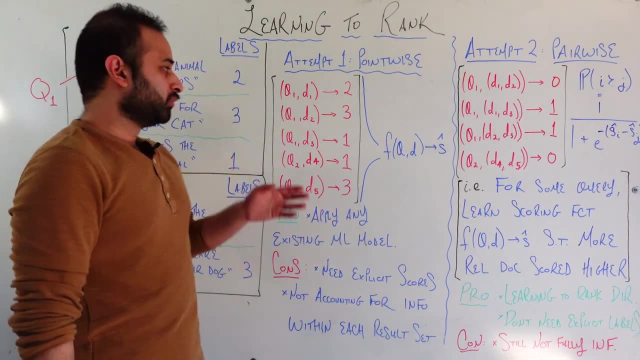 which is called the pointwise method. So our first attempt is pointwise. The pointwise method basically just calls each training example, so each sample in our training set becomes a pair of query and document. So we have query 1,, document 1,. 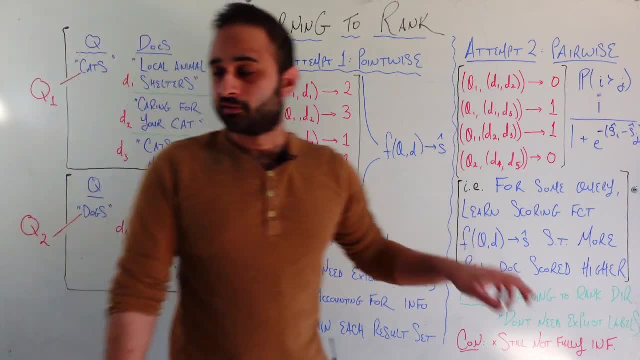 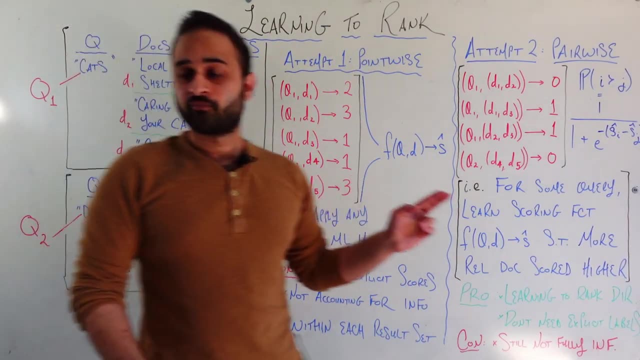 query 1, document 2, query 1, document 3.. That's these three documents and this query. And then we have query 2, document 4, query 2, document 5, and that's these two documents for that query. So we have five total training examples here, And 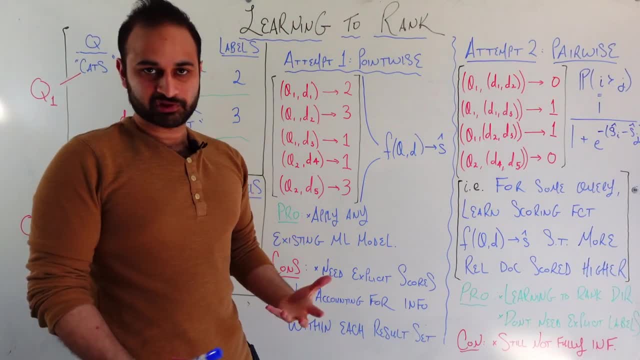 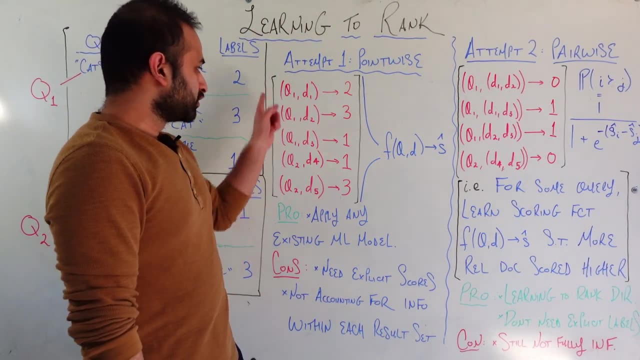 the labels for each one are simply just the relevance. So that's coming straight from this labels column behind me. here We have 2, 3, 1, 1, and 3.. And so for each pair of these guys we can derive whatever features we want to derive A couple that. 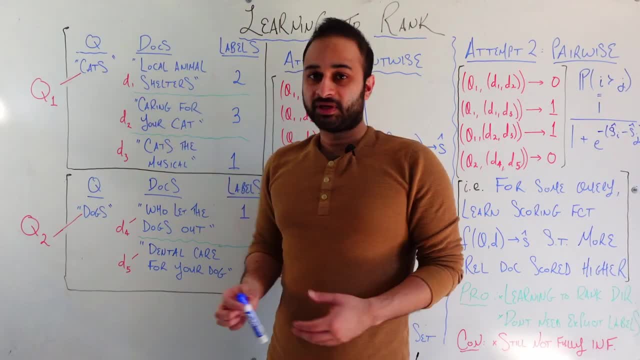 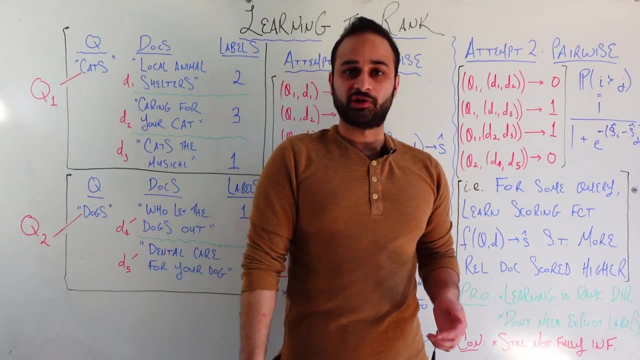 come to mind, for example, are, if you're looking at document-level features, maybe how many words are in the document or how many times are pronouns mentioned in the document. If you're talking about query-level features, then you could talk about how complex is the query. You can even have features that are kind of 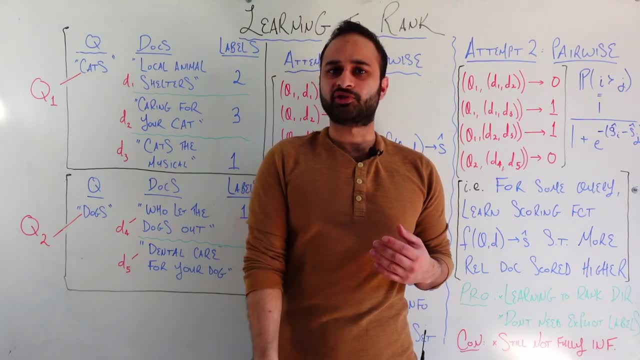 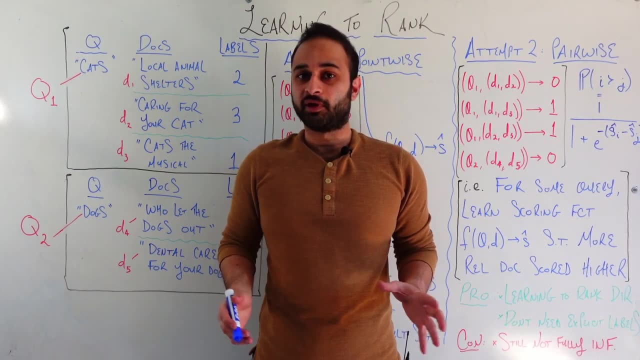 intersecting between your query and your document, like how many times does the word cats actually appear in each of these documents? So there's lots of different features, not the main focus of this video, but those are the features you'll be using in the model. So now we're starting to see how this is. 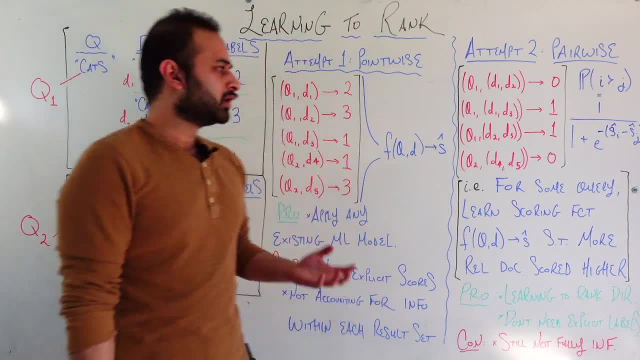 structured. So we're going to start to see how this is structured. So we're going to start to see how this is structured more like a traditional machine learning problem that we're all very used to. You have some features for each of these guys and you have 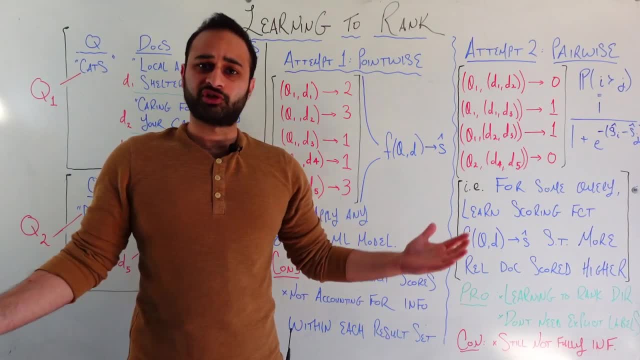 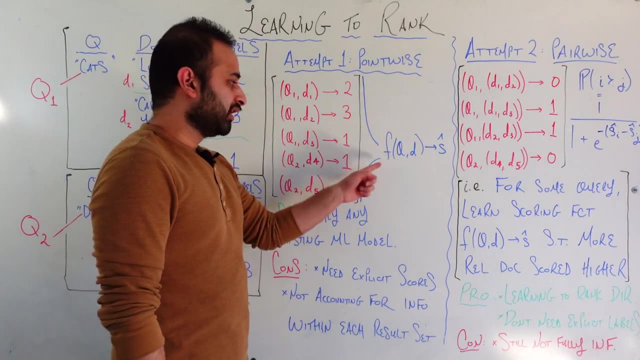 a label here. All that's left to do. you can apply your favorite machine learning problem, For example. we can use a regression or a classification problem in this case, and you'll just get a function at the end of the day that takes in a query, takes in a document. 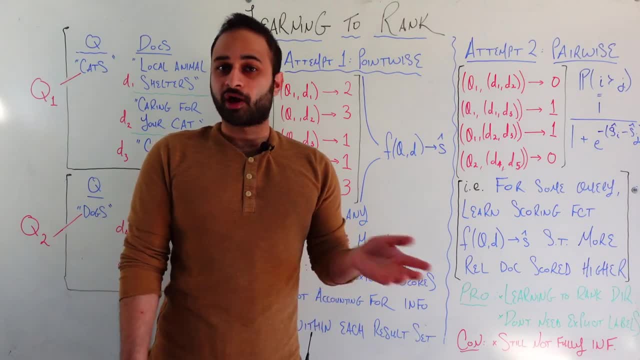 uses all those features derived from those guys and outputs some predicted score s-hat, And so this seems like a good approach to the problem. Why don't we just do this? If we can apply any machine learning problem, we can apply a function that takes in a query. 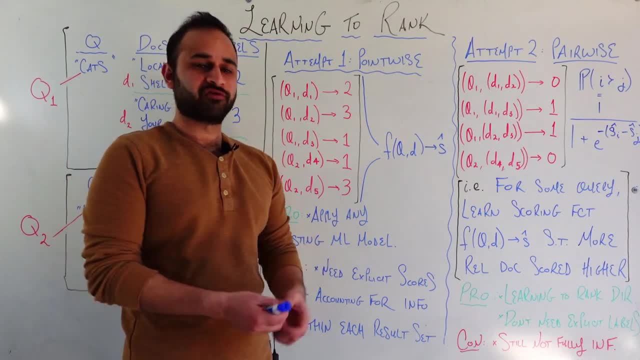 or a classification problem. So we can apply a machine learning algorithm that we've learned to this problem instead of having to derive some new math. Well, the pro is obviously that we can apply any existing model. You can just apply any model that takes in features. 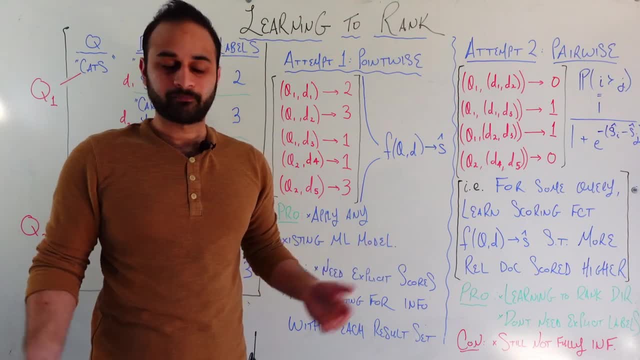 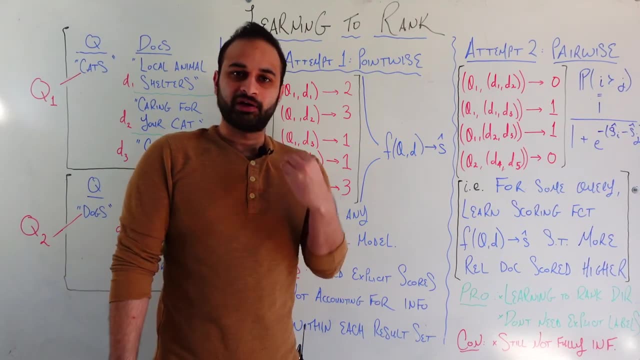 and is able to predict some kind of score. We have tons of those at our disposal, But let's talk about why we don't use point-wise models for learning to rank typically. We are missing out on a very important element here. We are missing out on the fact that 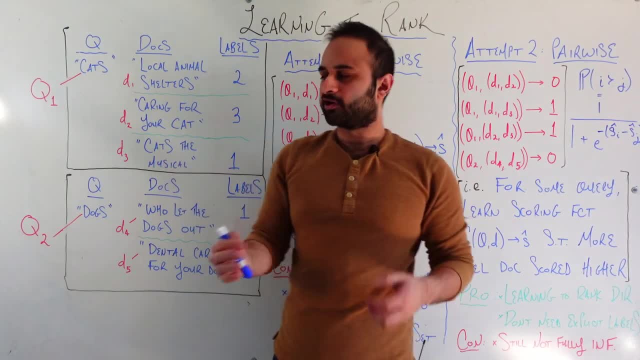 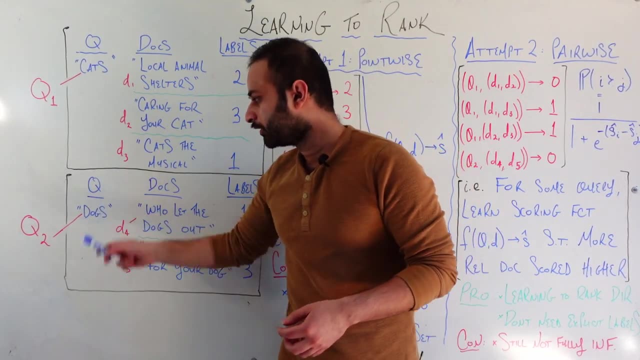 queries and documents have a very interesting relationship. For example, these three documents in some sense are tied to this query And these two documents here are tied to this query And by framing the training data in this sense, we lose all that information. 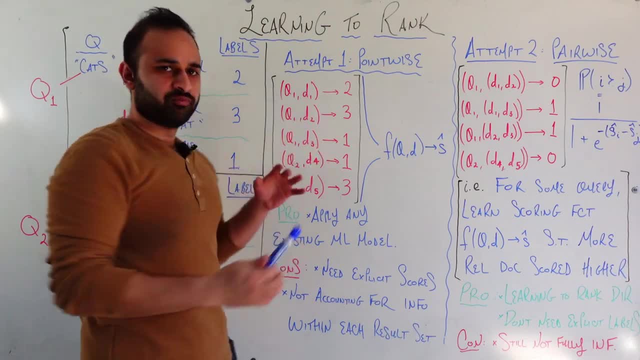 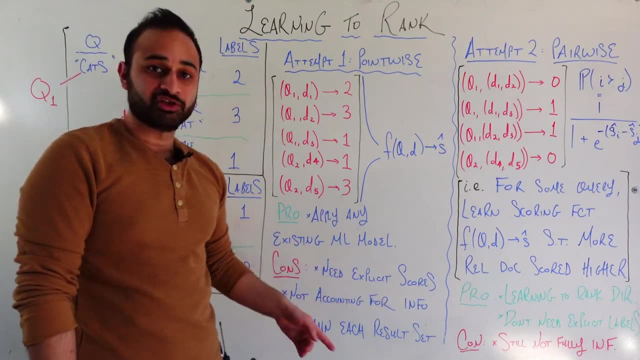 We lose this information, that this query and these three documents kind of belong together because we're just throwing them as examples in our data set, And so that's what we're trying to get at here- is we're not accounting for the information within each result set. 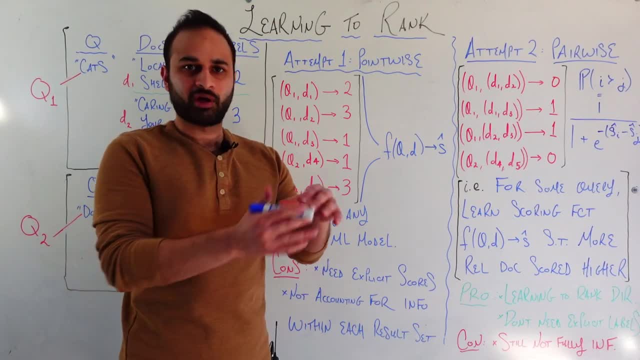 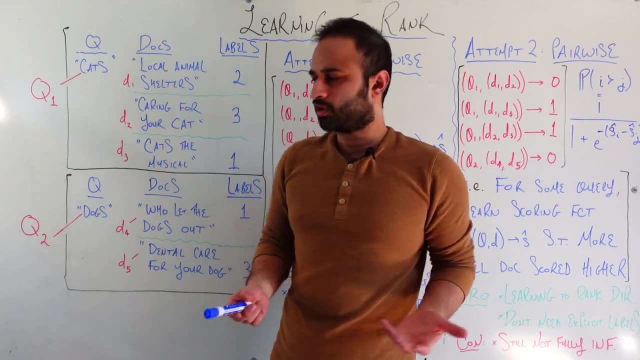 Because when you search for something, you're only really worried about the searches that are showing up right now. If you search for cats, you're very interested in these three results. If you search for the ordering of them, you're less worried about what could have showed. 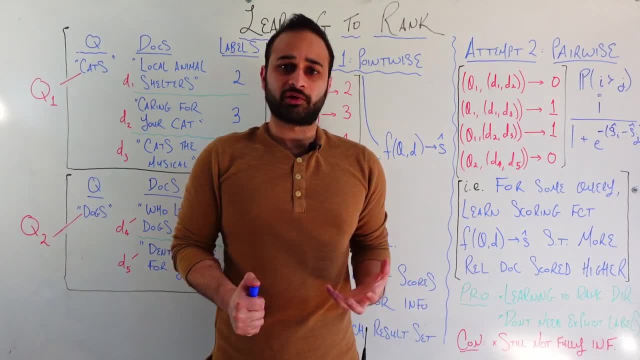 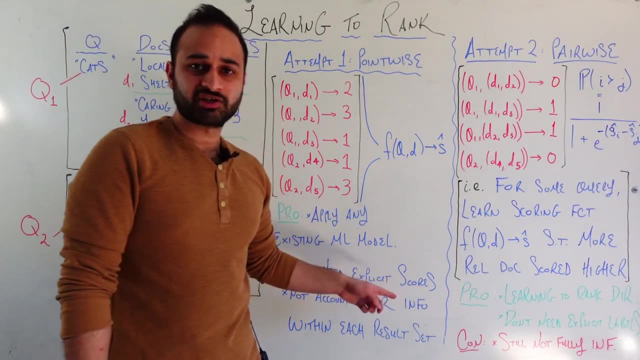 up if you searched for dogs. So that's why this point-wise model is not strong for learning to rank, But it is a good starting point. The other issue here is that we need explicit scores. As we were talking about before. these labels could be a little bit tricky to grab accurately And we need these labels in order. 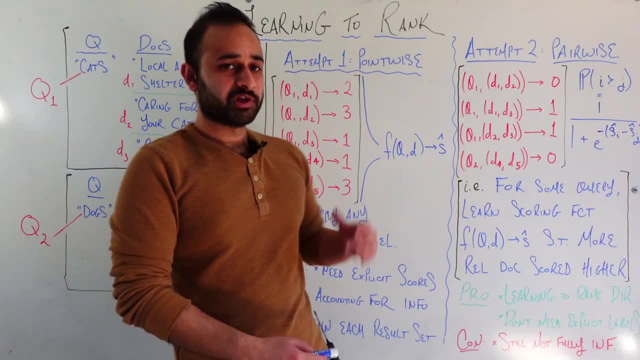 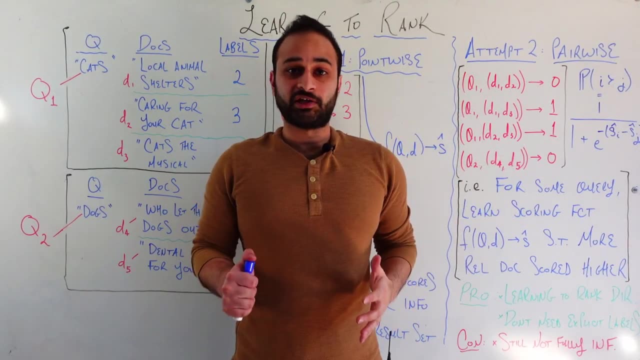 to use the point-wise method, So that could be a limiting factor as well. Let's move on to the next step of this learning to rank, which is the pairwise method. So the pairwise method finally starts taking into account the fact that certain documents kind of belong. 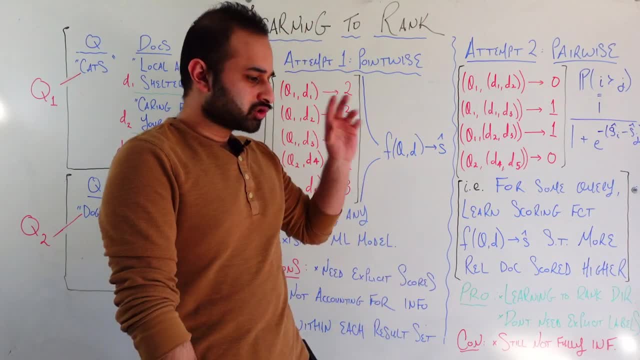 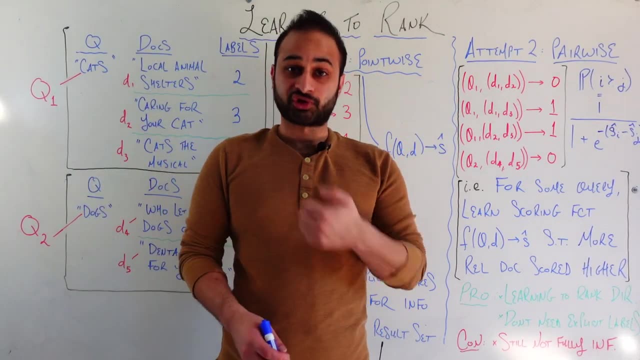 or are tied to certain queries, And let's see how it does that. So this makes a very interesting use of training data. Instead of framing the training data like this, we frame the training data as queries and pairs of documents. So, for example, if we're looking 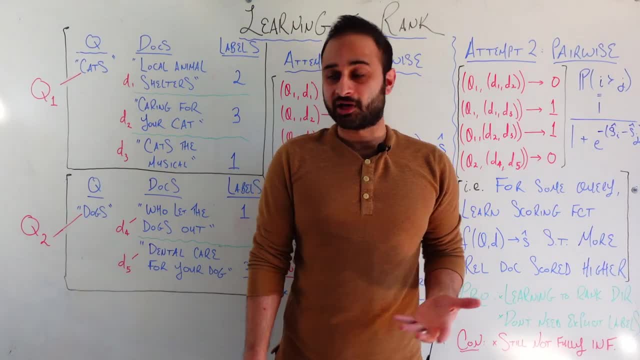 at query 1, what are the total number of pairs of documents we could have? We could have D1, D2.. We could have D1, D3.. We could have D2, D3. And those are the exact three things. 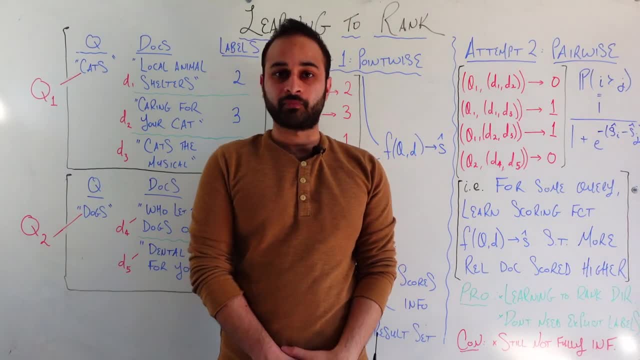 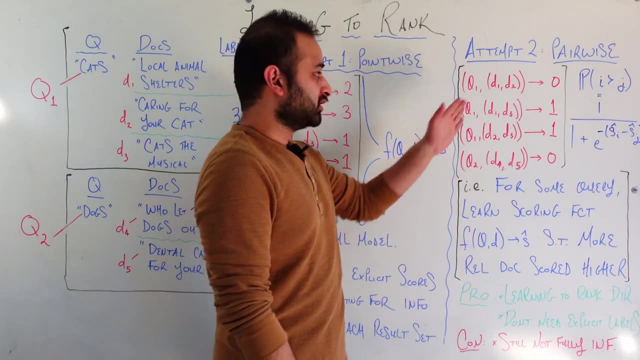 you're seeing as the first three examples in this training data. And what are the labels in this case? The labels are binary in this case And it's simply just a label that says whether D1 is ranked higher than D2, has a higher relevance. So we see that D1 is not. 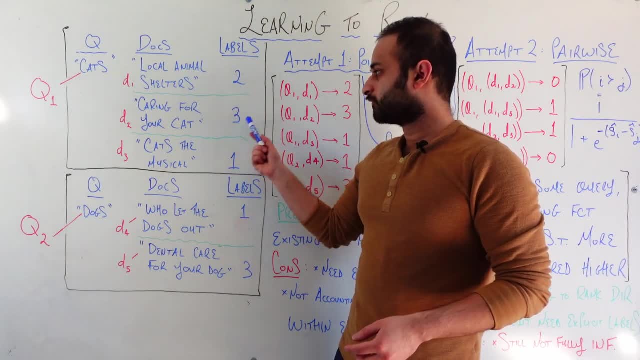 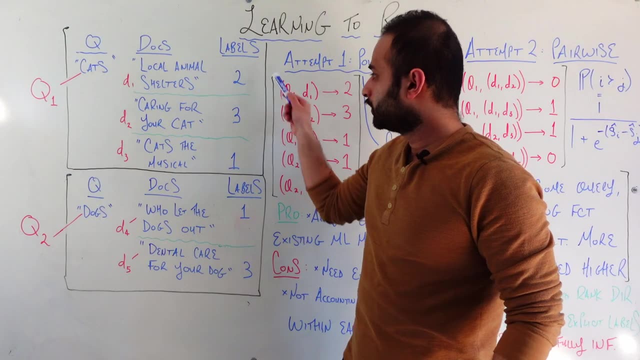 ranked higher than D2.. It has a label of 2.. This one has a label of 3.. So it's less relevant than 3.. Therefore we put a 0 here. D1, D3.. If we look at D1 and D3,, this guy does have. 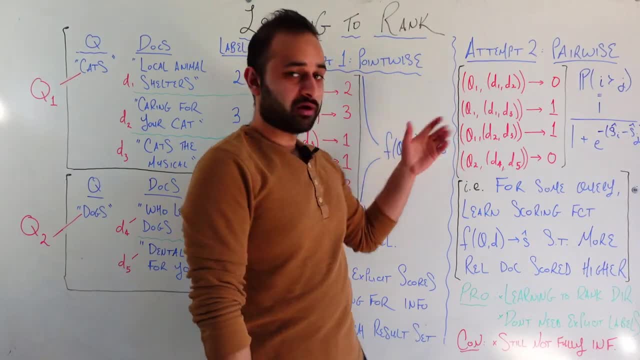 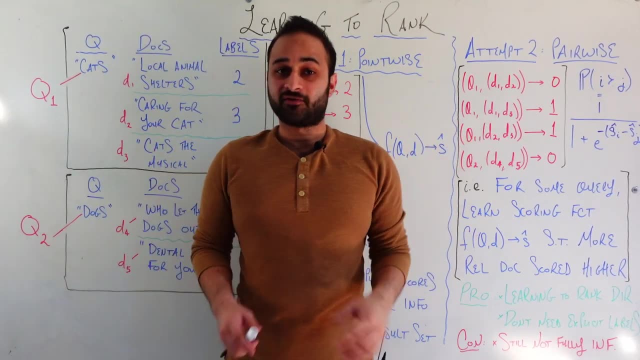 more relevance than this guy, So we give it a label of 1. And similarly for all these guys. So the fundamental difference, the main fundamental difference of going from point-wise to pair-wise, is that first we're framing our training data not as just independent samples. 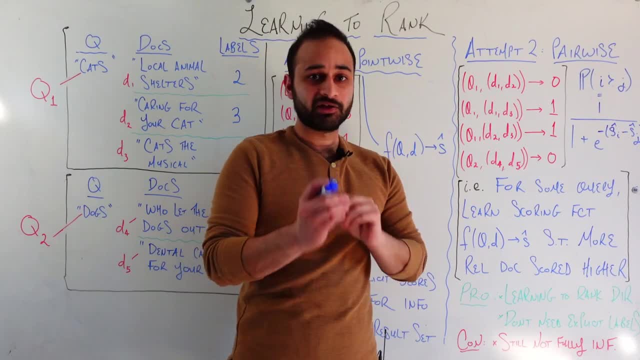 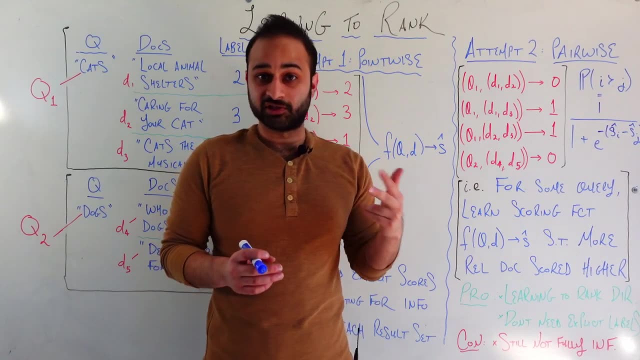 but as pairs of things that are within the same query. So we're inherently starting to take into account these very interesting relationships between pairs of documents and, specifically, their relevances versus each other for each query. So that's what we're seeing here. We're 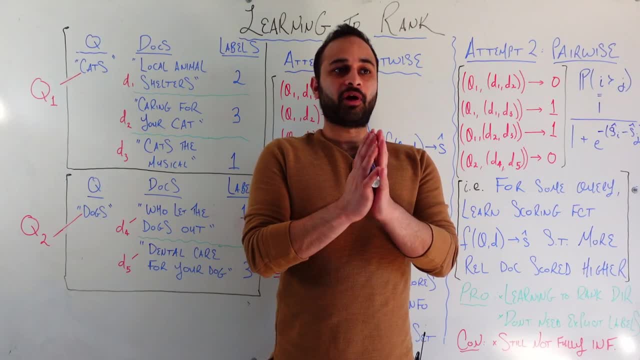 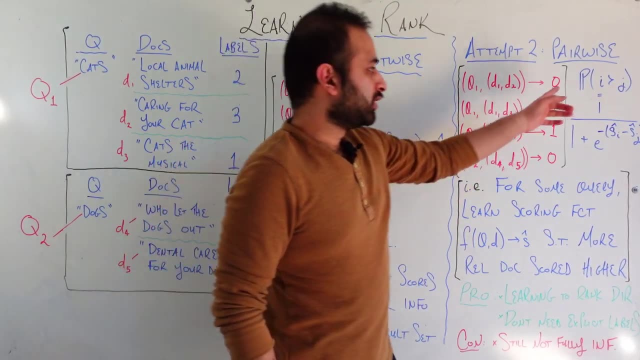 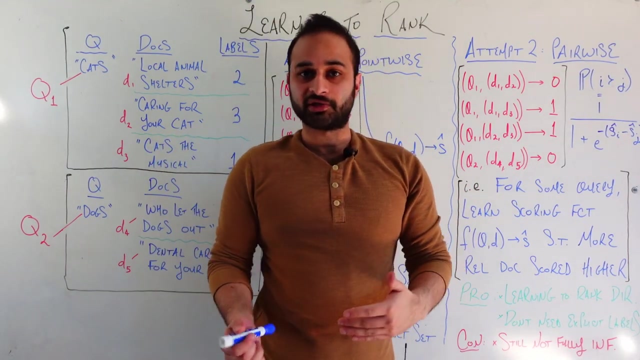 seeing here. The next place this differs is that now we are going to explicitly try to achieve the goal of matching the following probability. So here's some notation: PI, this weird little greater than symbol, actually means that I is ranked higher than J. So in 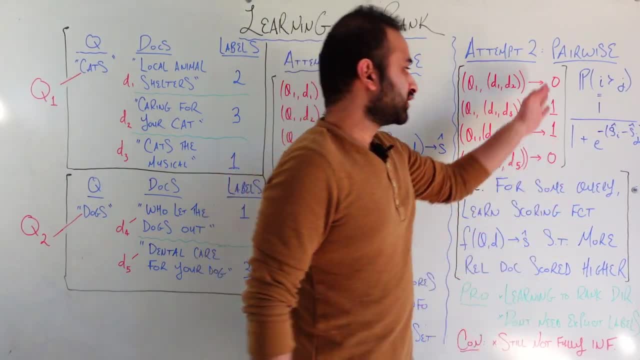 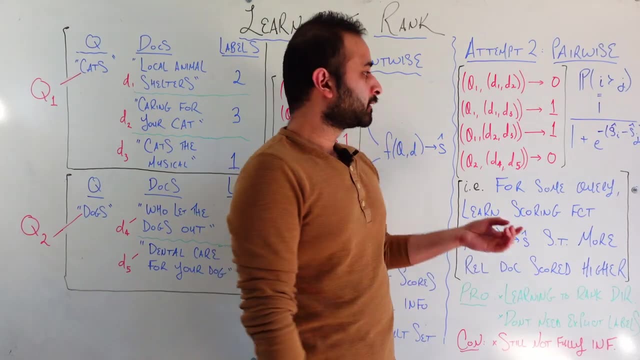 this context, I and J are some documents, And this term here means what's the probability- that document I is ranked higher than document J for a particular query, And we're going to model that as this, This very common form that we've seen before, the sigmoid form of 1 over 1 plus e to the 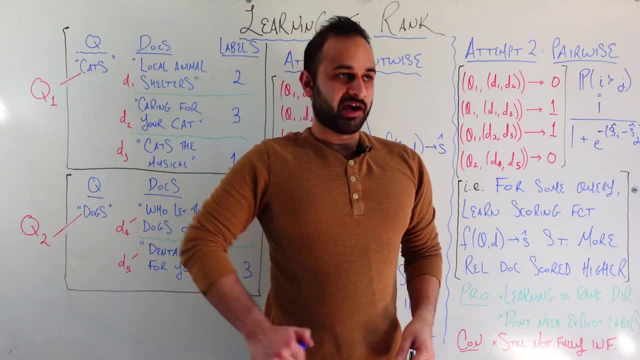 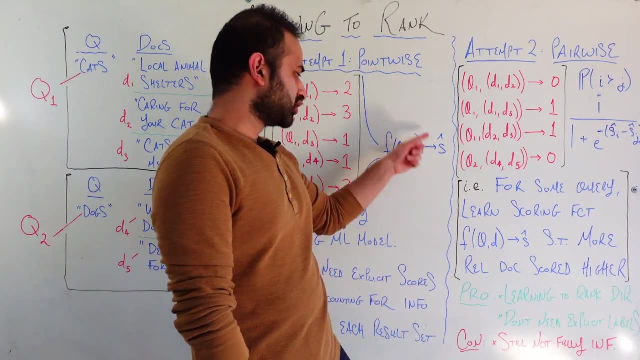 negative SI hat minus SJ hat. I think this deserves a little bit of explanation because you might be a little bit lost here. But what's going on explicitly is that we're still trying to learn some kind of function, just like here, which is going to take a query and a document. 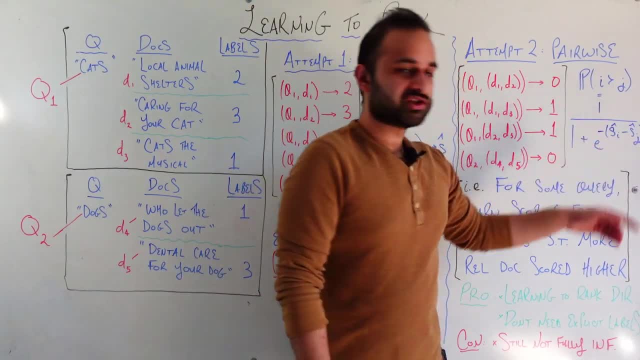 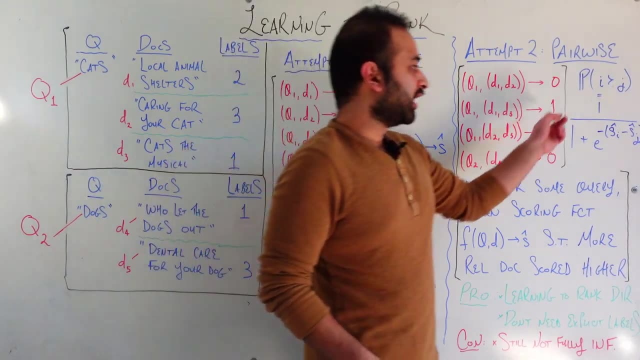 and output some kind of score. That score is SI, SJ, hat and so on. But instead of treating these scores independently, as we were doing in the point-wise model, we are going to be directly trying to optimize or match this probability. To be explicit here, for example, let's say: 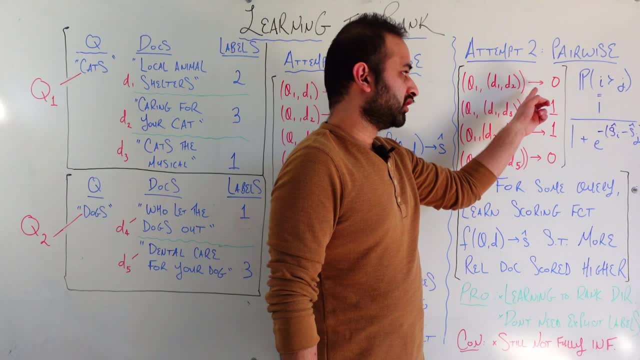 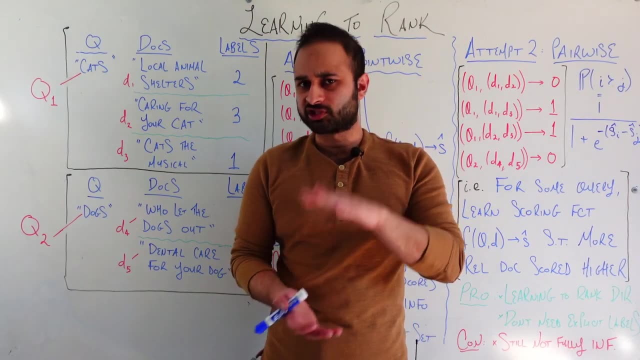 that we're looking at document 1 and document 2.. We know that the label here is 0, so this probability should be very small. because we want the probability that document 1 is more relevant than document 2 to be very small because in honesty it's not. It has a label. 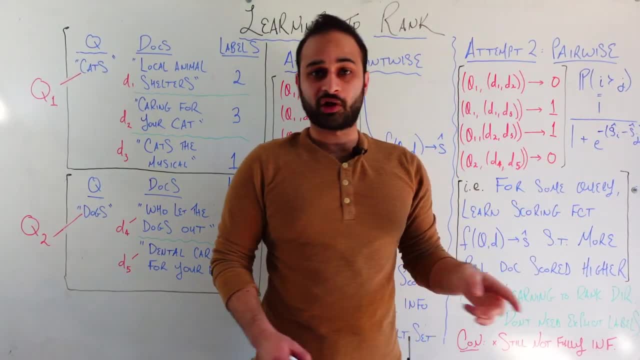 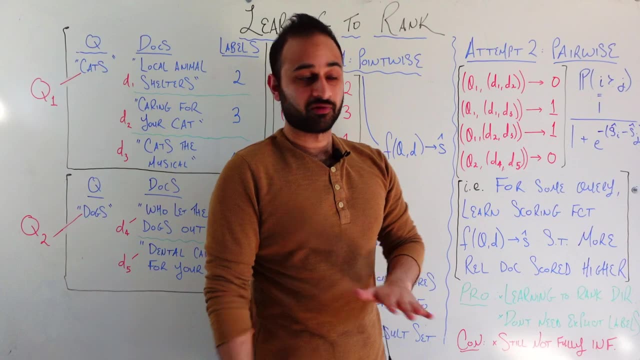 of 0.. So we're going to try to find some kind of scoring function such that this probability for these two documents here is as close to 0 as possible. Conversely, if we're looking at the document pair D1 and D3, we're going to be looking at the probability that this 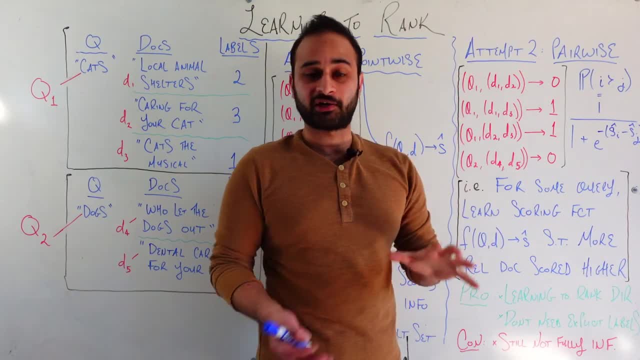 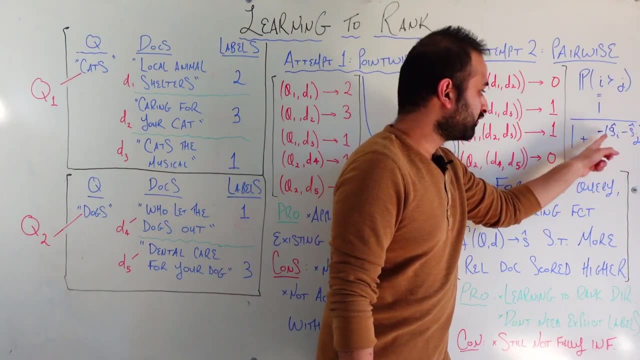 is 1.. So, in fact, if we're trying to find a scoring function for the document P3,, we want this probability to be as high as possible because, in fact, document 1 is actually more relevant than document 3, has a label of 1 here. Therefore, we're going to try to find a scoring function. 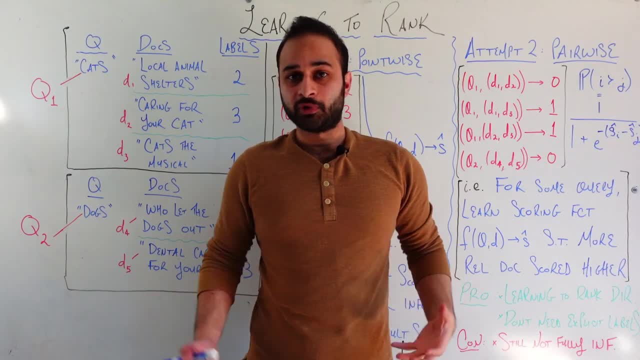 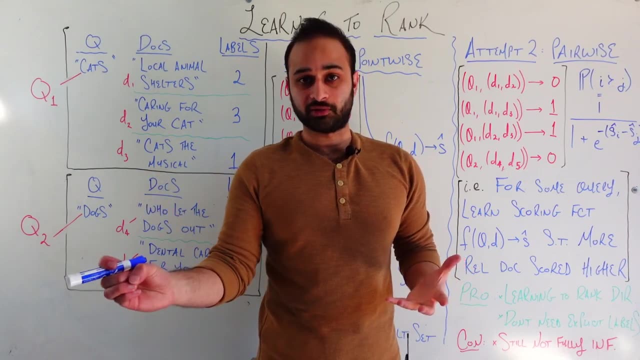 such that this form becomes as close to 1 as possible. So I'm kind of masking some of the details here. I didn't want to go too deep into the map. but behind the scenes we are trying to find a scoring function so that the scores that this thing outputs are gonna. make these probabilities match as closely as possible to the actual truth in this table. We are going to test it out and see if we get any real results. Then we're going to test it out and see if we get any real results. So we are going to test this out and see if. 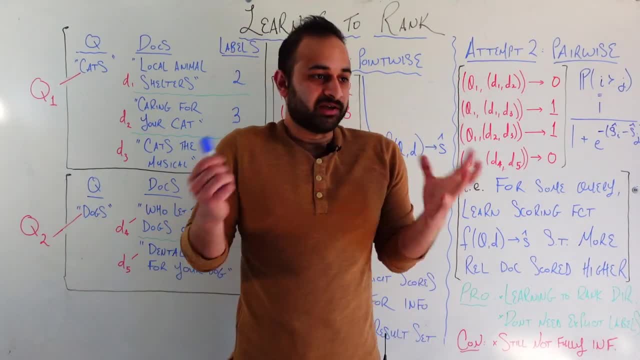 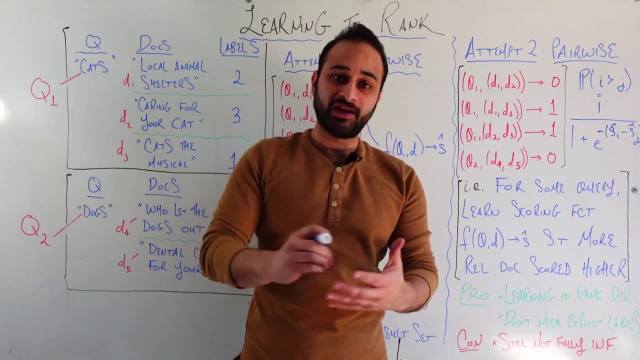 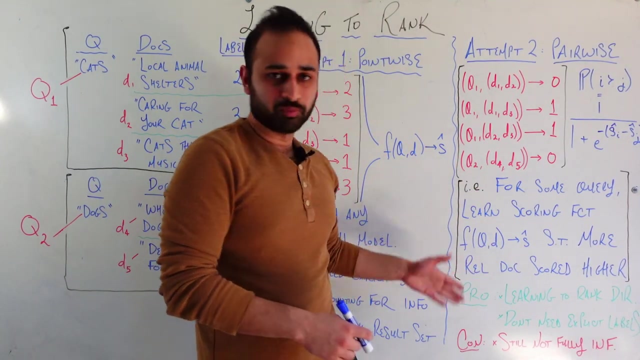 to the actual truth between pairs of documents, and so this whole idea about certain documents being linked to a particular query, certain documents being more relevant to others, given that query, is baked into this model, which is not true for the pointwise method, and so everything i said is kind of coalesced into this blurb here. the pro here is obviously that we're directly 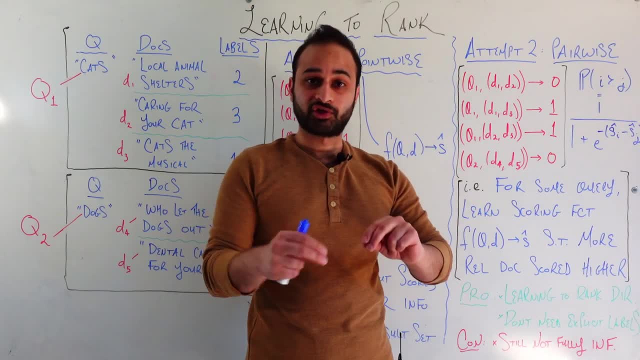 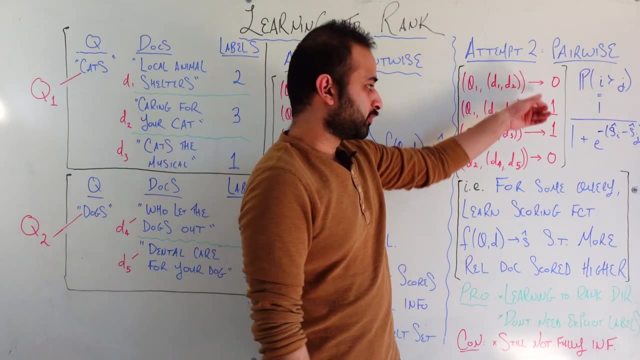 learning to rank. here we're taking the relative rankings directly into account in the model. the other pro is that we don't need explicit labels here. for example, notice that our labels are just binary, so we don't need to know what the actual ratings here are, we just need to know. 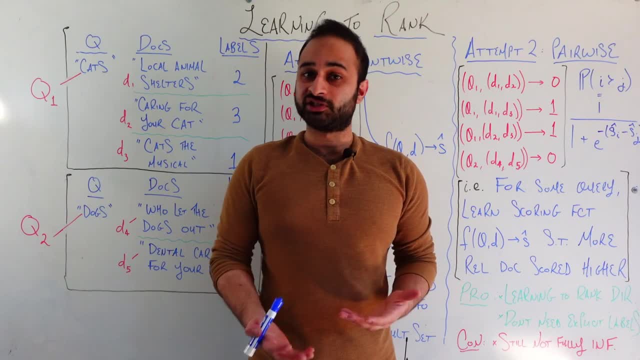 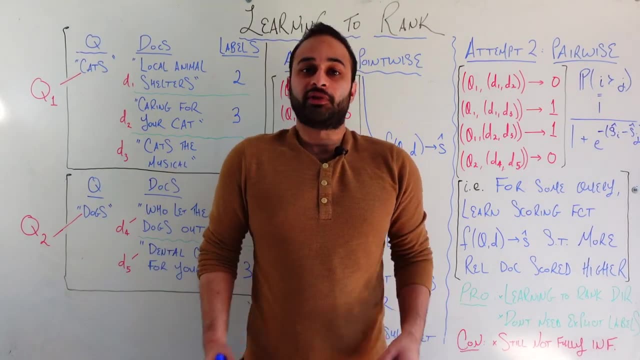 whether one rating is higher than the other. that can be a big win in many situations where it's hard to get these labels. the con here is that, believe it or not, this model is still not fully informed, even though we have begun to take into account these relationships between documents in 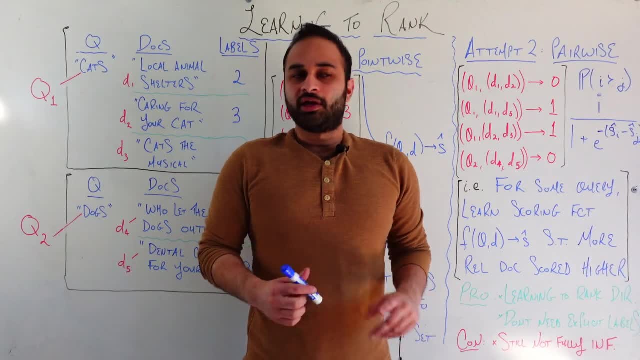 the same query. we're just doing it in a pairwise way. if we wanted to do, you know, if we wanted to do a pairwise way, we would just do a pairwise way. if we wanted to do a pairwise way, we would just do a pairwise way. if we wanted to do a pairwise way. 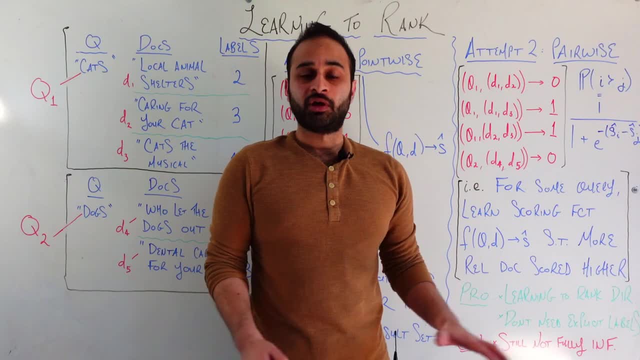 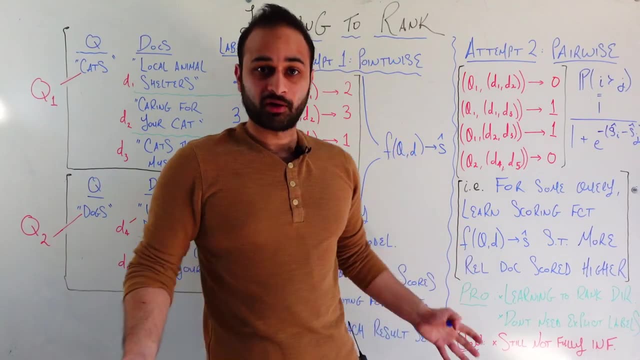 this in an overly powerful way, in the best way possible. we would consider all of these documents for a particular query at the same time, and that, even though i ran out of room here, is the next step. so those are called listwise methods, and i've chosen not to talk about them here because we've 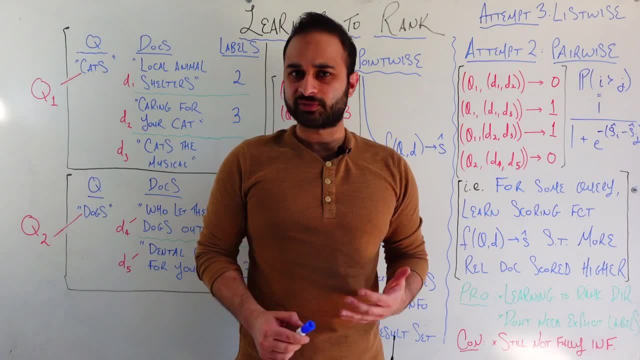 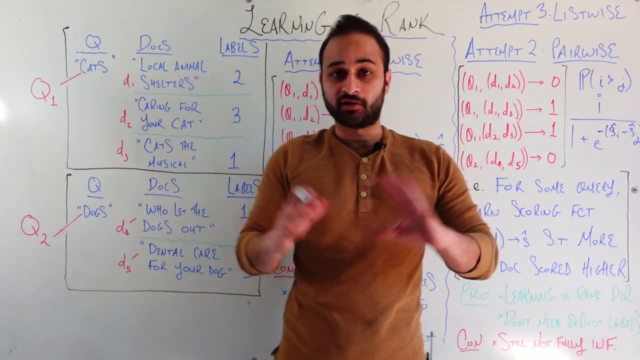 already talked about a lot in that video. if you want to talk about listwise methods, let me know in the comments below. but they are one step further and they basically take into account the entire set of documents at once, not in a pairwise fashion, but just all of them together. 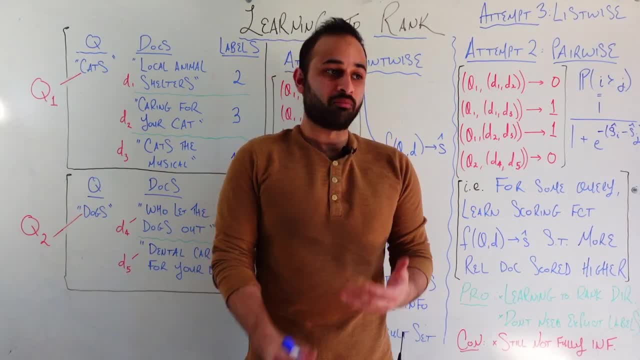 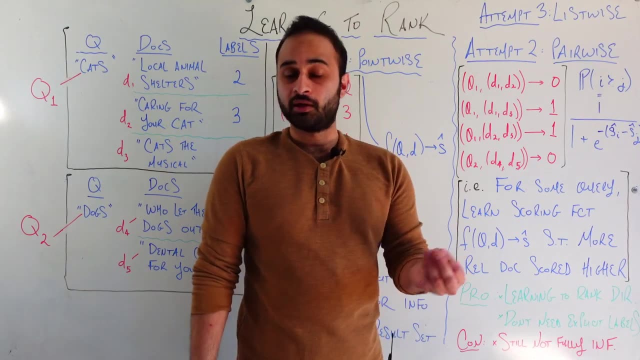 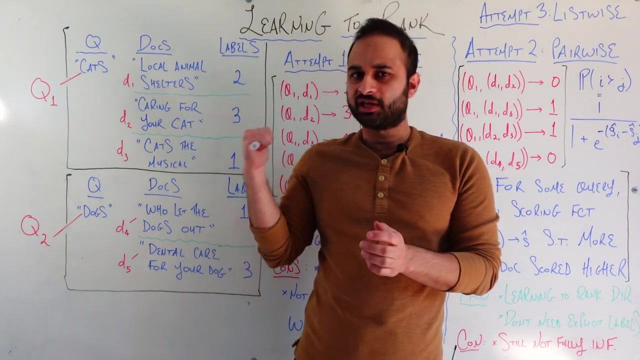 so the pro of them is that they do this in a more theoretically sound way. the con is, of course, you might have guessed, they're very complex. you have to do them in an efficient way in order to do it at all. so hopefully you learned how we do, learning to rank, starting from this naive, pointwise method. 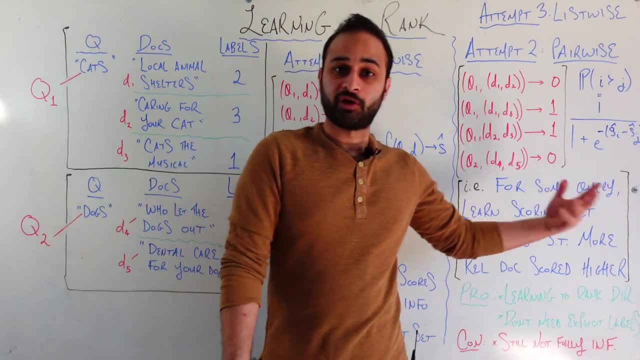 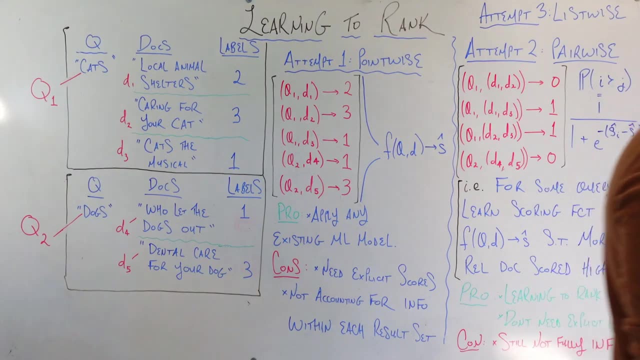 talking about why it doesn't work, talking about this pairwise method and moving beyond that. so if you learned something in this video, please like and subscribe for more. just like this, and i'll catch you next time you. 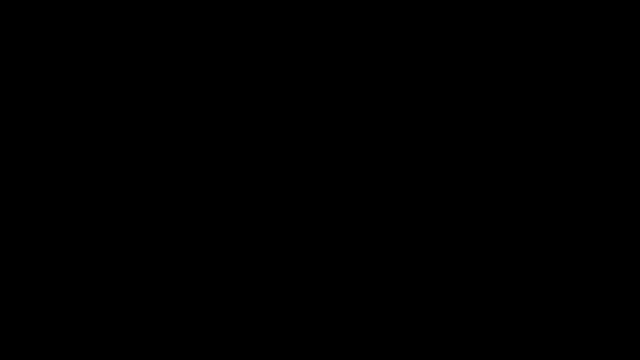 In this video we're going to talk about how to graph polar equations. These include circles, limousines, rows, curves and lemniscates. So let's start with a circle. The first equation you may see is: r is equal to a cosine, theta. 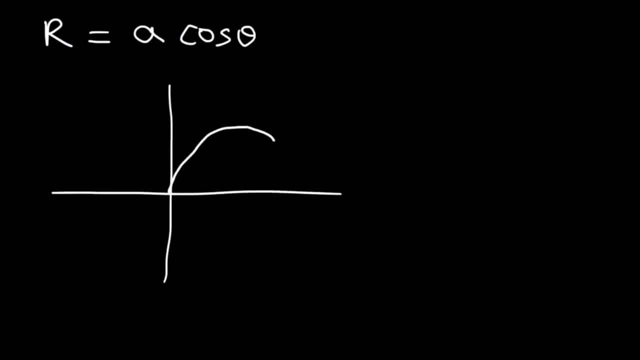 Now, if a is positive, this is going to be a circle directed towards the right. Now, granted, my circle is not perfect, so bear with me. A is basically the diameter of the circle And this is going to be the center of the circle. so if you go up to find this point here, it's half of a.